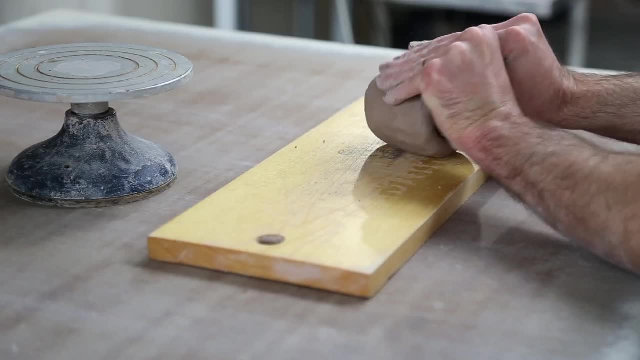 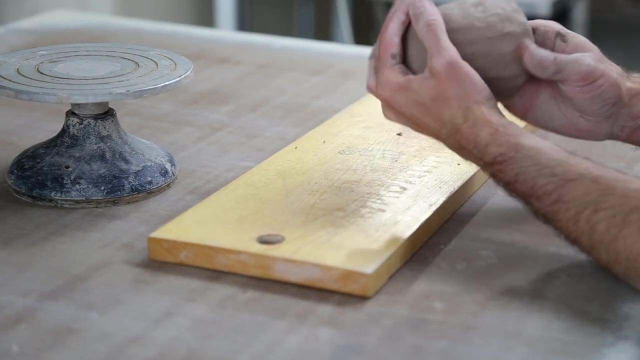 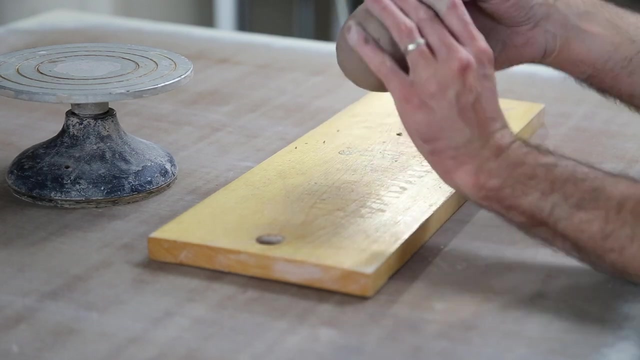 come out. Thinness is kind of the end goal here, because if the walls are thick we're going to end up with a heavy object, and we don't want a door stopper, we want a fully functional utilitarian object. So down at the very bottom of the pinch pot there's some thick clay that I couldn't quite. 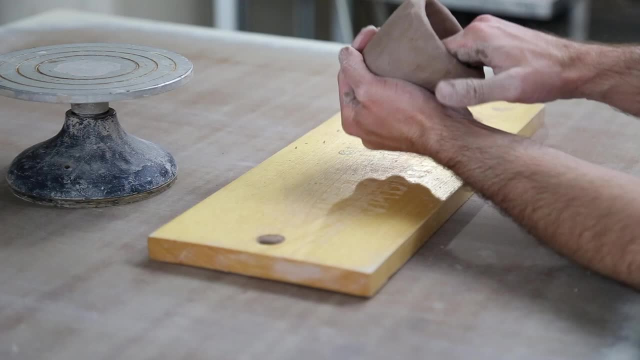 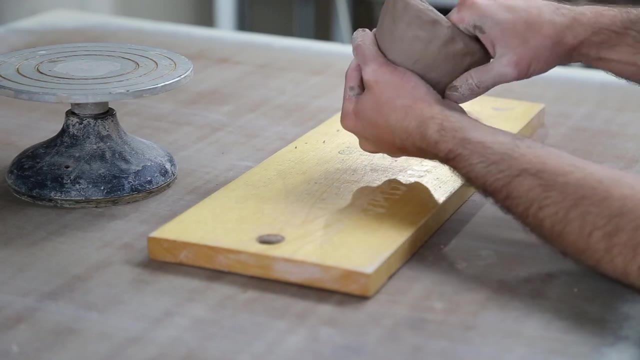 reach with my thumbs. so I'm supporting the base of the pinch pot with the palm of my hand in a cup-like motion and just kind of compressing down with my fingers of my right hand. This is going to make the pinch pot conical or cone shaped down at the very bottom, but that can be pretty easily. 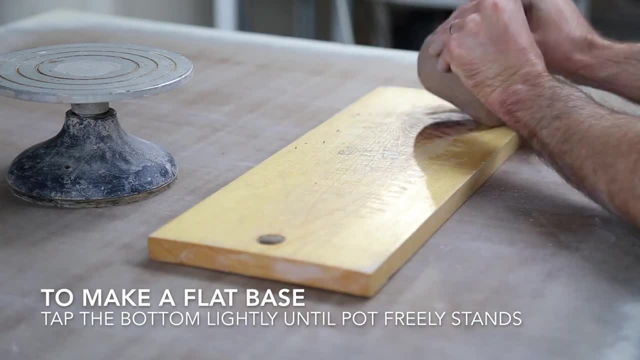 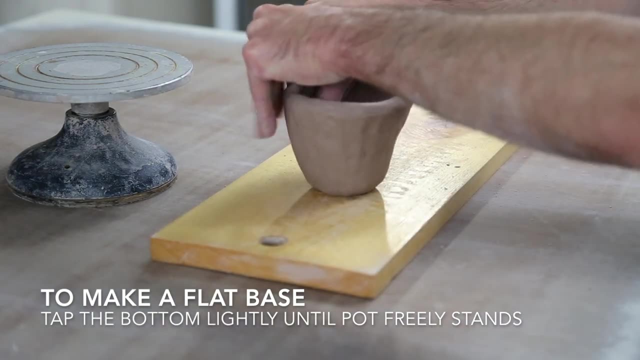 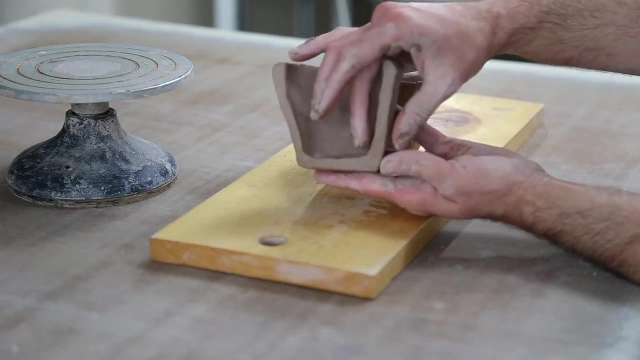 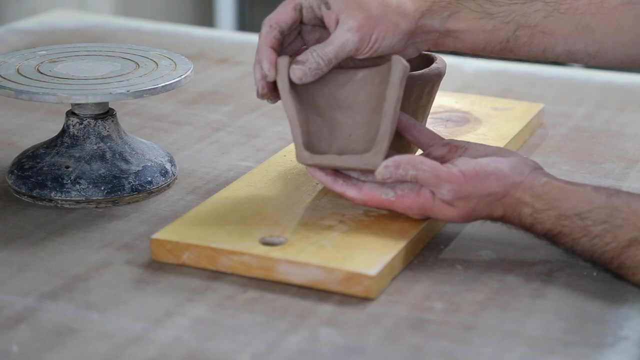 fixed by tapping the base on the table or adding a foot ring. All right, now you can see the walls are adequately thinned out. so now I can take this time and shape my pinch pot, trim the rim and kind of smooth out the surface so that it looks a lot better. 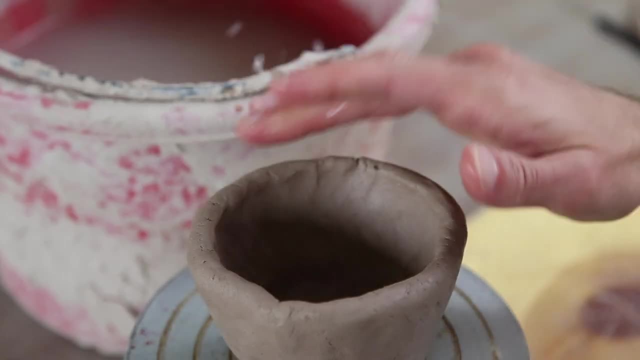 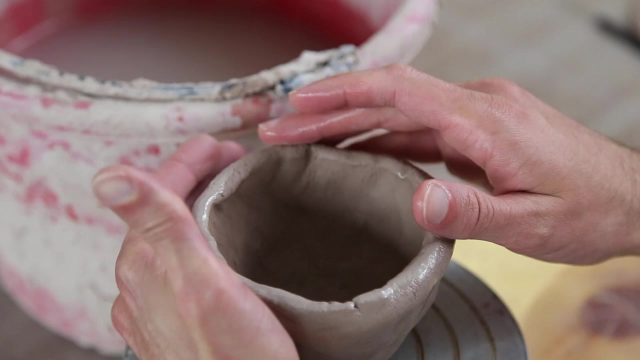 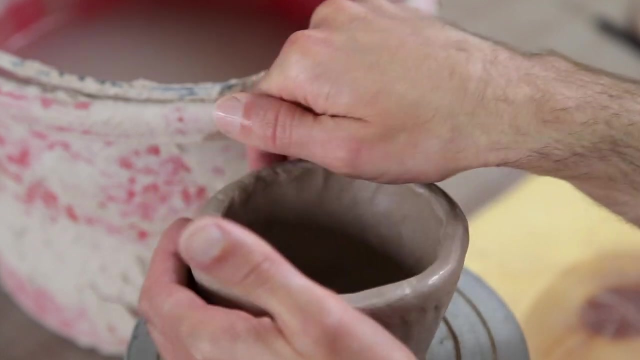 If, while you're making your pinch pot, you're noticing the rim cracking, simply just add a little bit of water to the rim and smooth it out. Just a dab will do. It'd also be a good idea to kind of gently compress down on the rim, and that'll really make sure that the clay platelets. 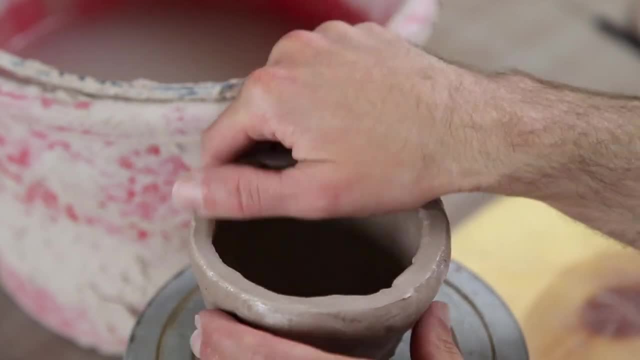 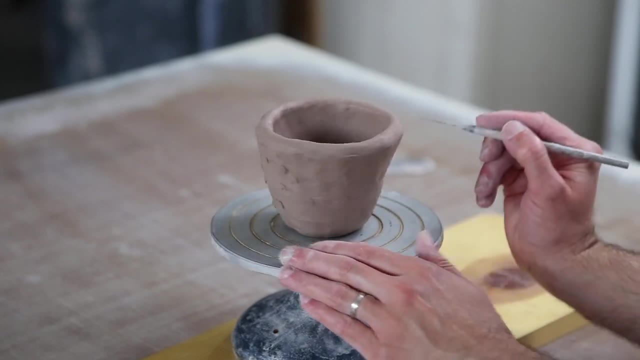 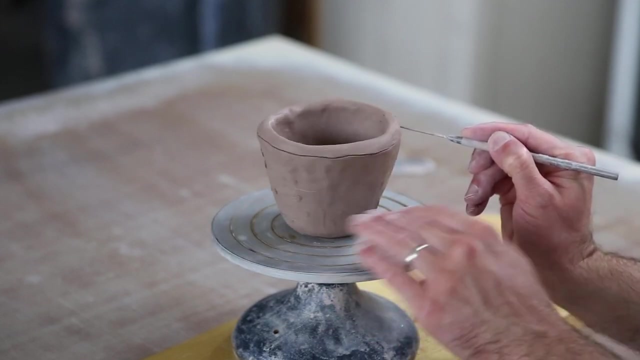 fuse together so that you can avoid more cracking in the future. So now I'm going to trim the rim of the pinch pot level. What you're going to need to do first is center the pinch pot on the banding wheel or a kick wheel, or any wheel for that matter, and with a needle tool or a scalpel. 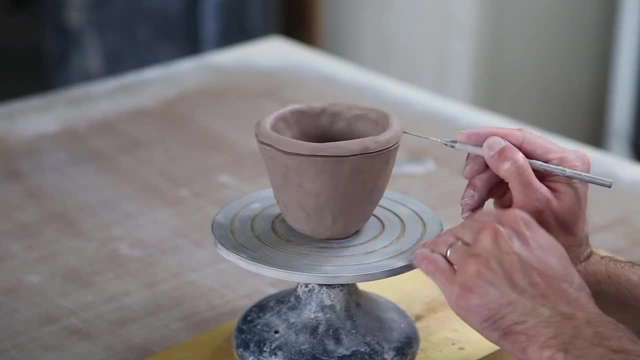 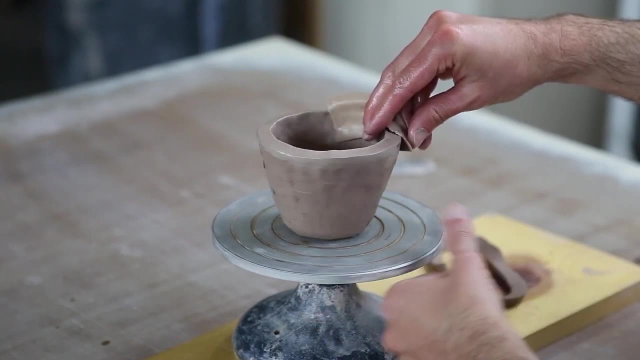 draw a line with a steady hand at the very top where you intend to cut. You might need to make a couple pass throughs, but gently lift off the excess amount that has been cut away and then, with a sponge or a chamois, just smooth out the rim. 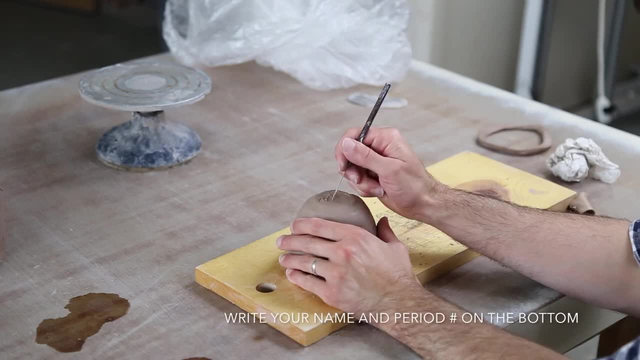 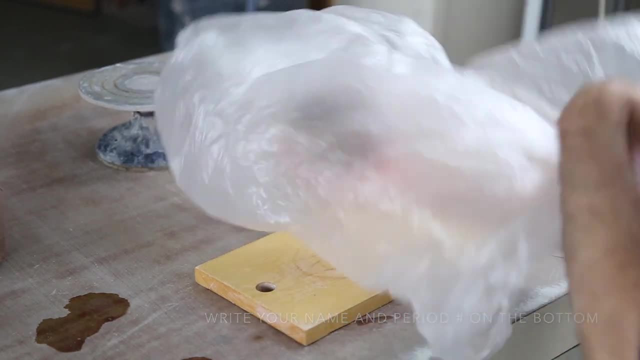 After you're finished on day one, you're going to want to turn your pinch pot upside down and scrape your name and period number on the bottom of the pinch pot. This is so you don't confuse it with anyone else's. Gently put it into a plastic bag- no need to spray it at this point- and cover. 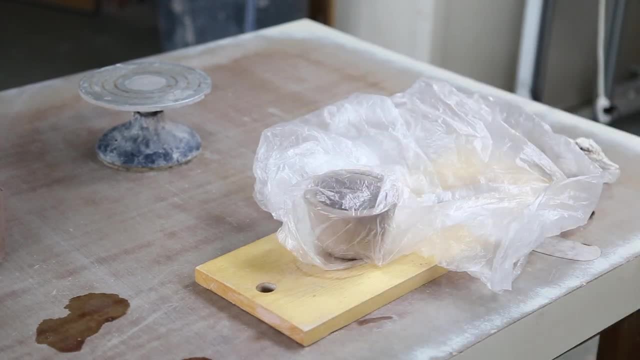 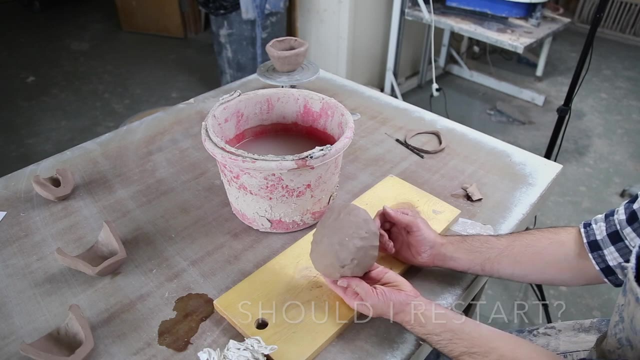 it up completely, Set it on a wear board and then gently slide it into your cubby space. So since we're still on the topic of day one, let's talk about a couple of things that could go wrong. Let's say your pinch pot isn't looking much like a pot at all. Let's say that it's flaring out too. 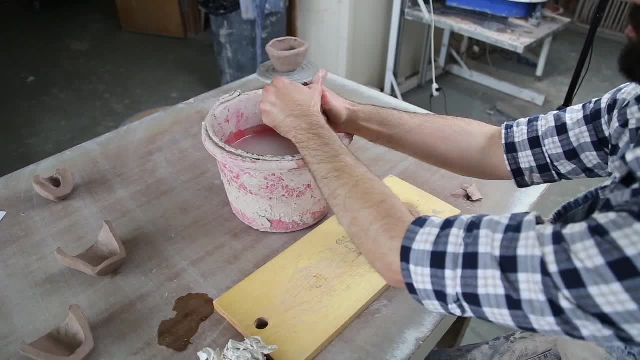 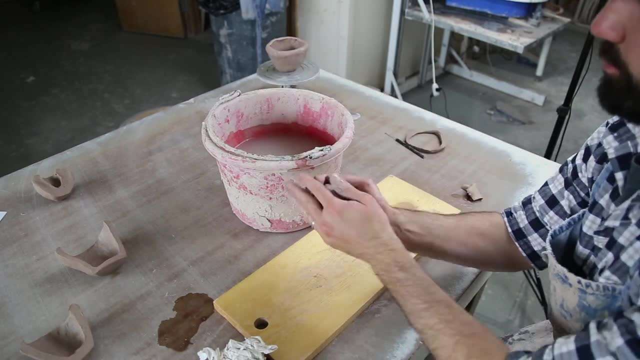 what you could do is take your clay and dunk it back into the water bucket that's at your table, Smash it in between your fingers multiple times, You could even try and re-wedge it, but ultimately just work it back to the normal pliable plastic consistency of the clay that you 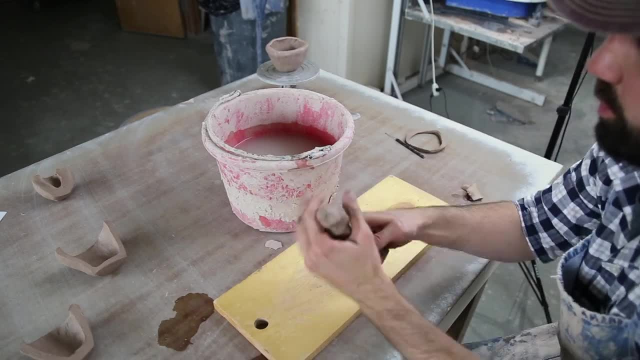 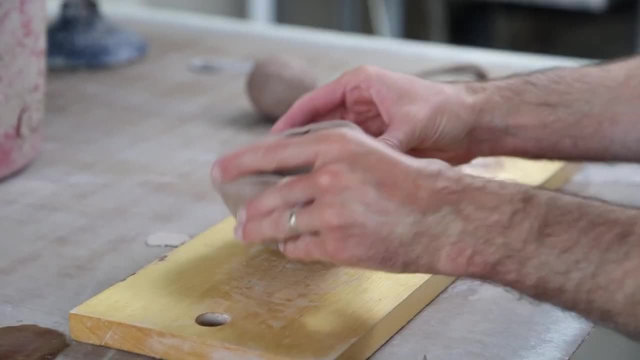 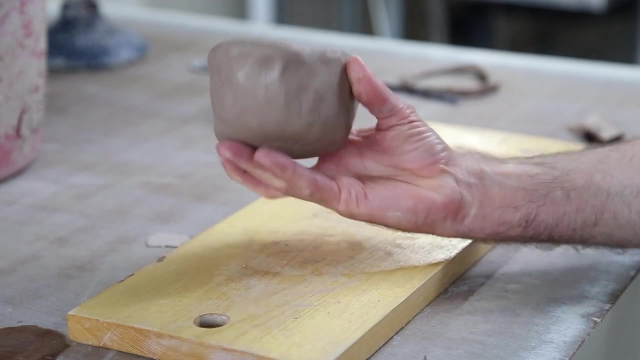 originally got out of the bin. Once that's done, the clay is ready to use again. Also, be careful with the way that you handle your pinch pot. You don't want to aggressively tap it on the table or mishandle it in any way That misshapes the overall form. Otherwise, that might likely. 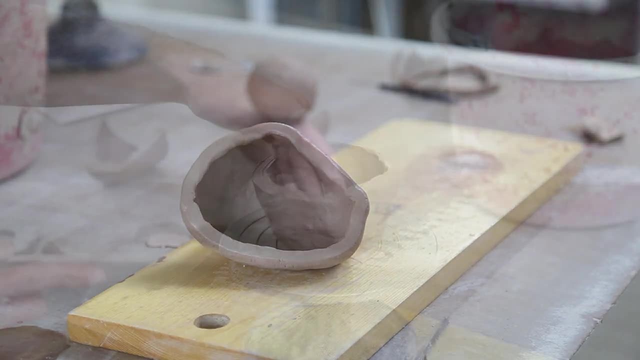 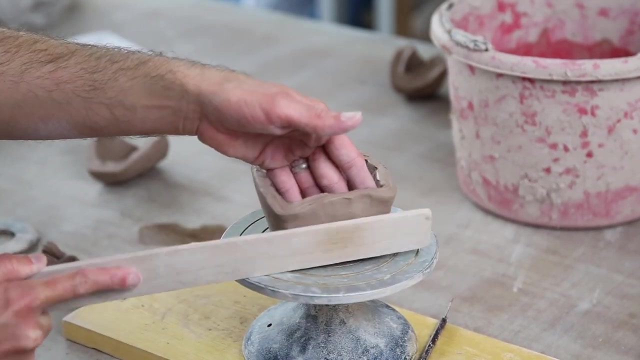 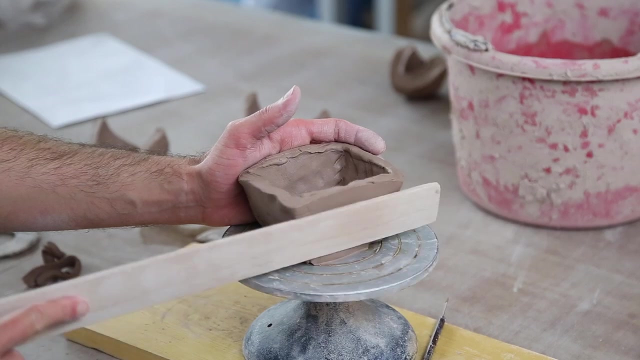 result in a restart, and that's never fun. If I'm wanting to alter the form in any way, that's going to come from the pressure that I put in certain areas of the pinch pot. So the square that I'm making right here, I've pinched the corners and I'm kind of pushing up against the inside base. 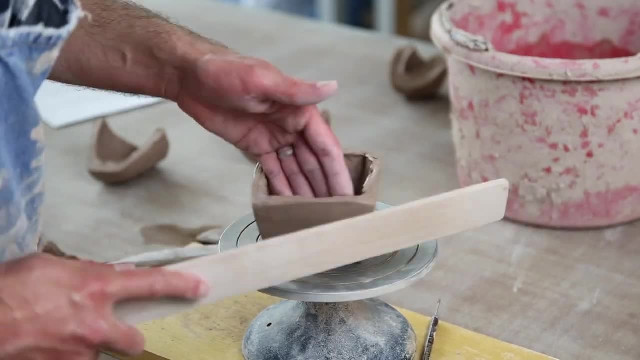 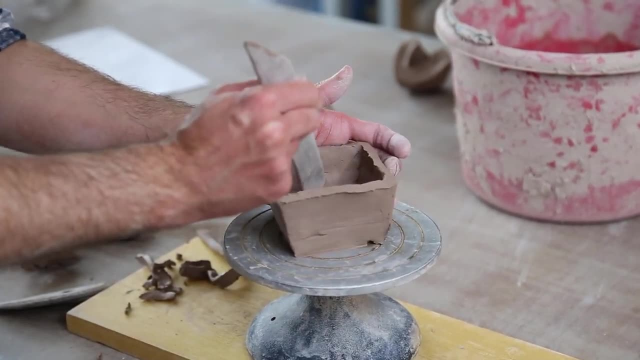 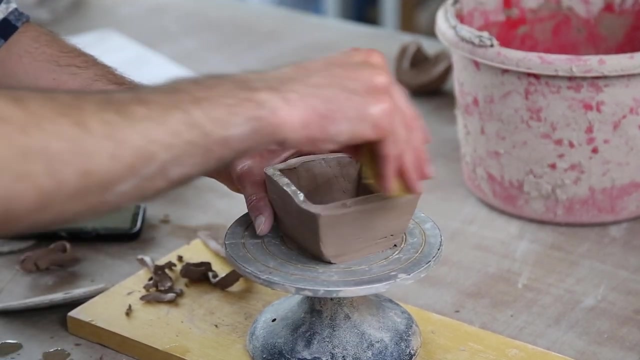 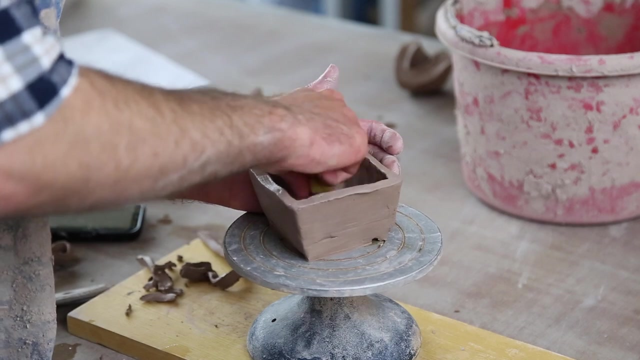 or the wall, excuse me with a finger. So pressure, counter pressure. Once I've pinched to make that kind of squared off shape, then I'm going to take a pedal and kind of just pedal up the sides to assist with getting that squared off form. Also, a trimming stick or a flat rib tool will help kind of smooth out the flattened surfaces. 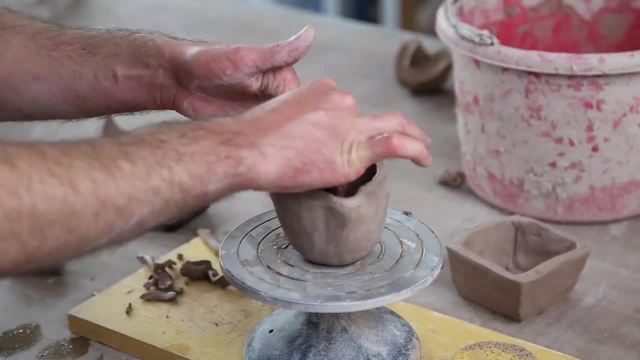 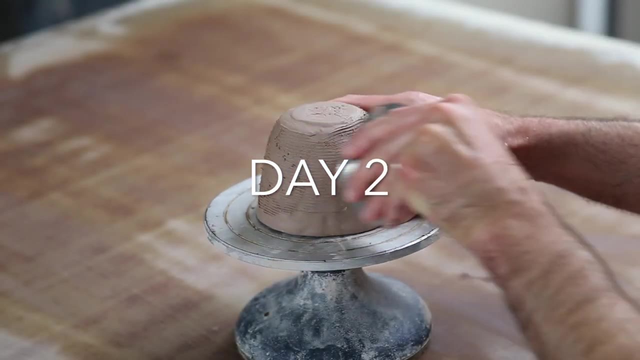 of the squared off sides that I'm trying to achieve. It takes a lot of work to get, but eventually it all comes through Alrighty. so on day two, remove your pinch pot from the bag and check to make sure it's leather hard. Leather hard is when the clay is. 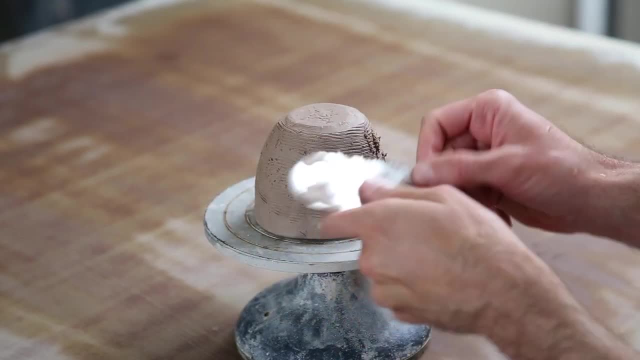 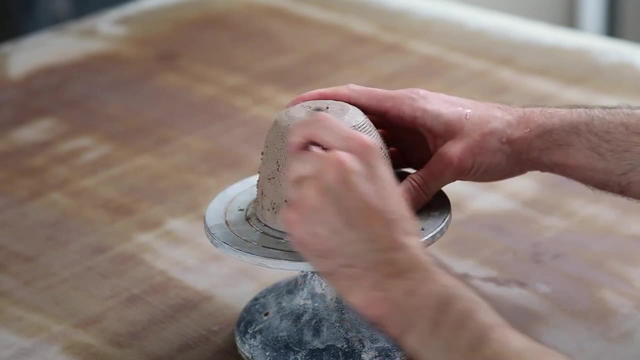 no longer plastic and durable enough to withstand the pressure you put on it. It shouldn't bend or flex very much at all. So what I'm doing right here- and one of the ironies of working with clay- is that you have to sometimes rough up the surface in order to smooth it out. That's very applicable. 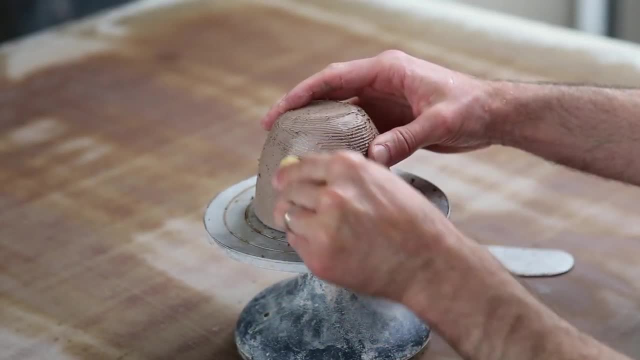 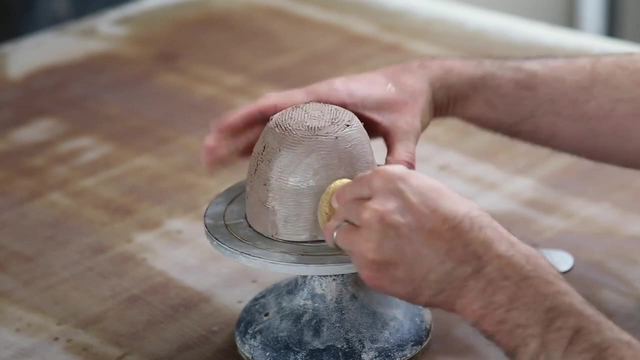 in this situation. If I want to eliminate my finger marks and indentations, I need to score the surface likely multiple times to achieve the desired effect. Then I need to smooth out the surface in a waxing motion with a dampened sponge. Yes, this will make the surface a little gruggy, but 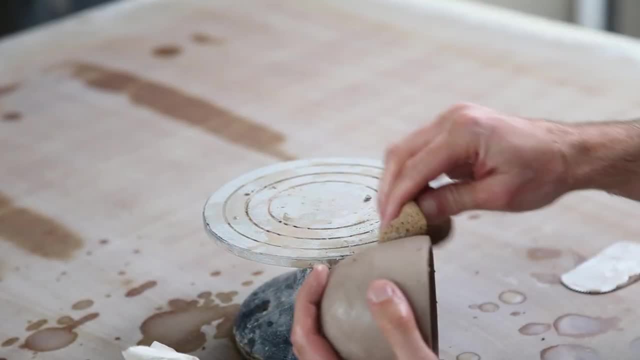 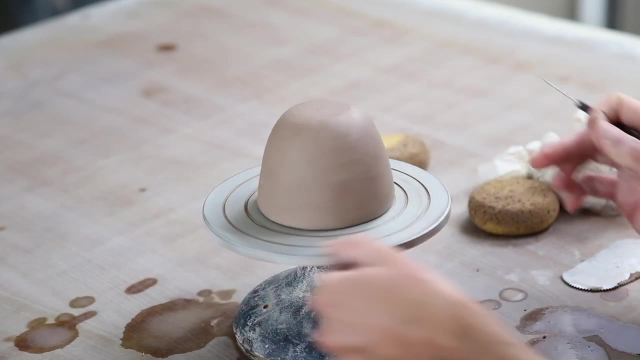 then I can burnish it down with the flat side of the rib or the back side of a spoon. Alrighty, so it looks like I'm done here, Just going to place this upside down on the banding wheel and spin it a few times to make sure that I've achieved the symmetry that I was looking for all through shaving. 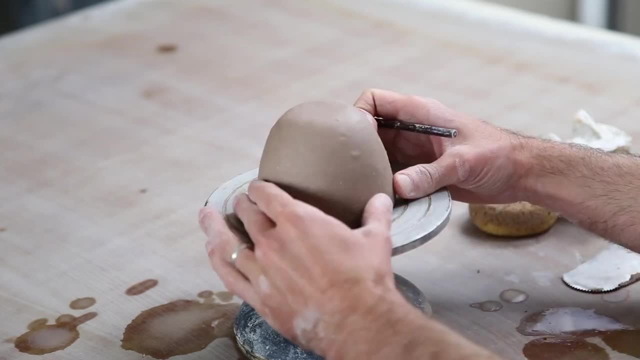 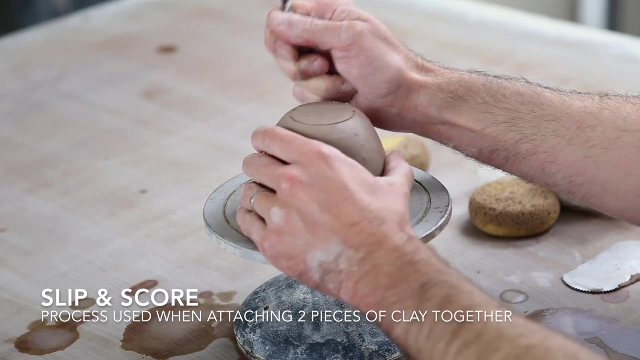 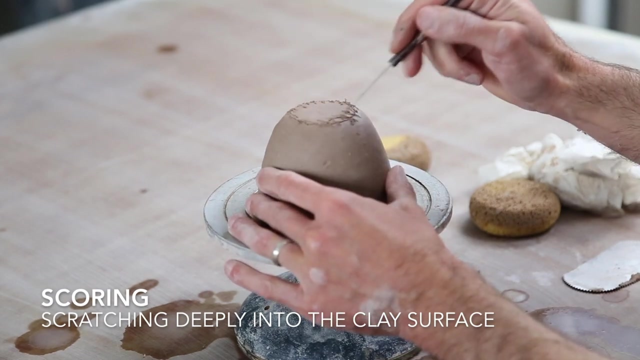 and paddling. So, after achieving symmetry in my shape and smoothing it out, I'm going to add an elaborate foot ring to the bottom of this pot. To do so, I'm going to place a small coil by slipping and scoring it into place. Scoring is the action of scratching the surface. you intend to add clay to. this allows. 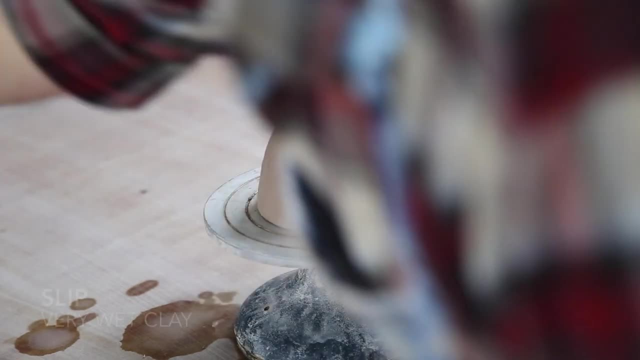 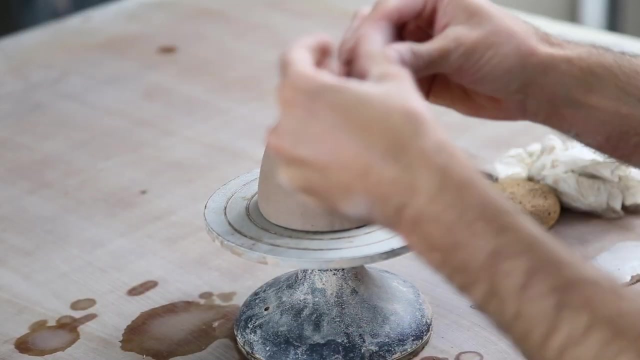 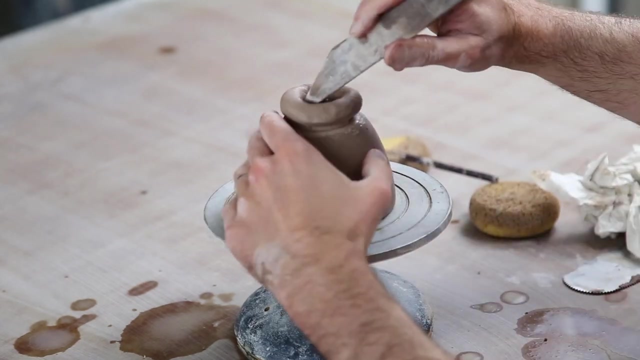 the platelets to readily interlock together. Slip is like the bonding agent that glues the clay together. These two actions assure that your two pieces of clay will stick together. I'm going to continue to pinch this ring down with my finger until it gets a little wider. Basically, just think about making it another pinch pot underneath your. 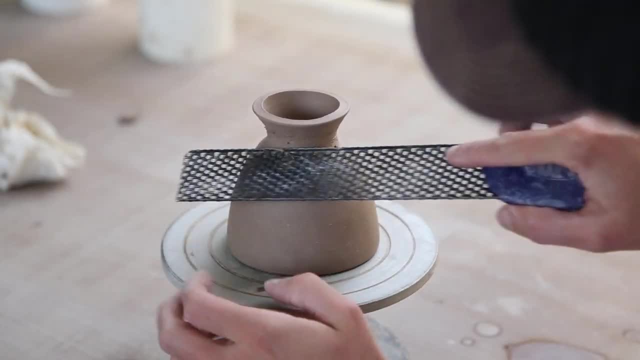 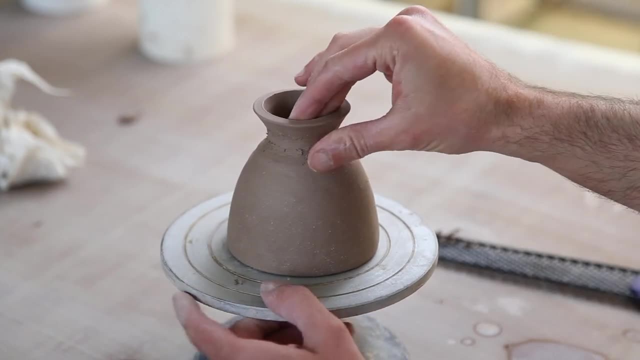 first pinch pot. So already I've pinched the foot, thinned it, trimmed it and smoothed it out. I'm going to take a rasping tool and square the area where I attached the ring and then I'm going to smooth it out with a sponge for a seamless transition from the body to the foot. 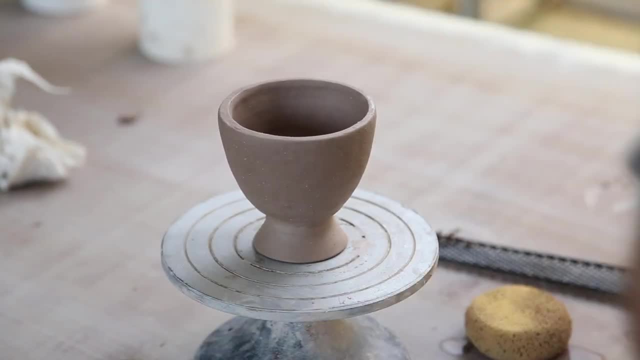 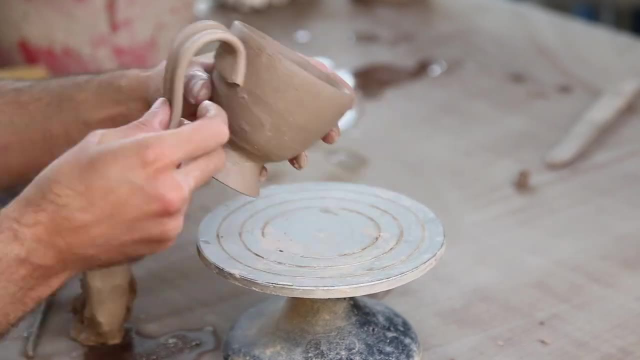 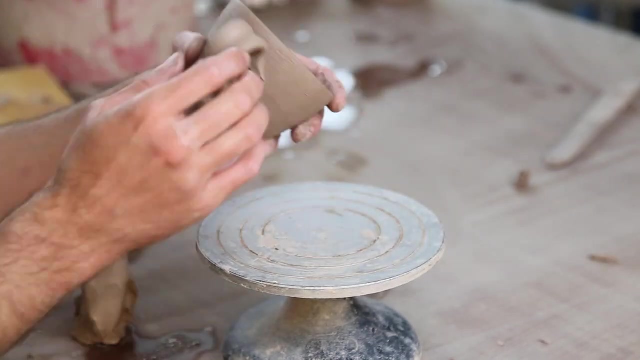 Next, I'm going to add a handle to the pinch pot. Not that it needs one, but I feel like it'll suit the form and will likely be more aesthetic than utility. Just like when I attach the foot ring, I'm going to slip and score the handle to the side profile to assure that it sticks well on the pot. 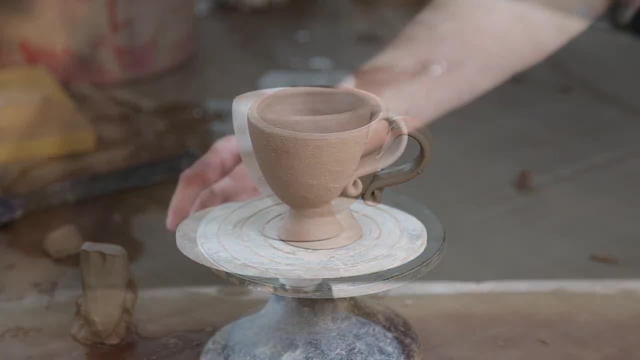 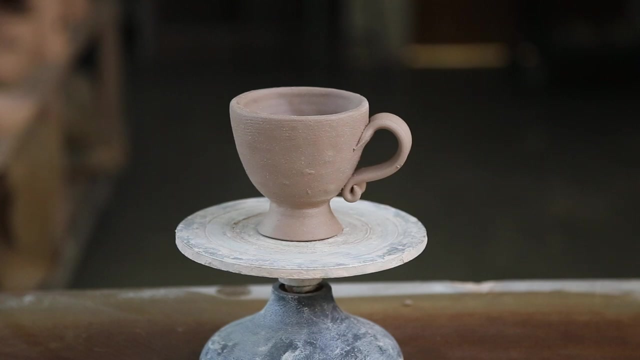 And that, my friends, is how you make a pinch pot. Thanks for watching. Have you any idea why?